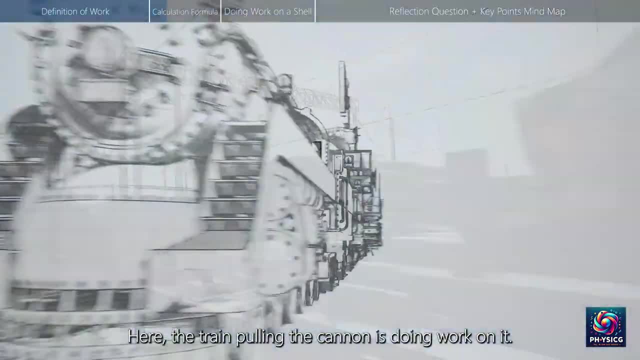 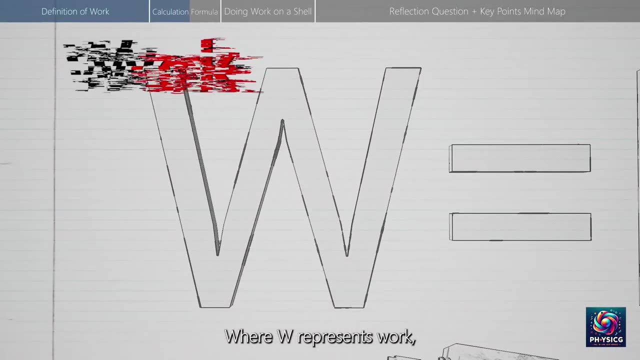 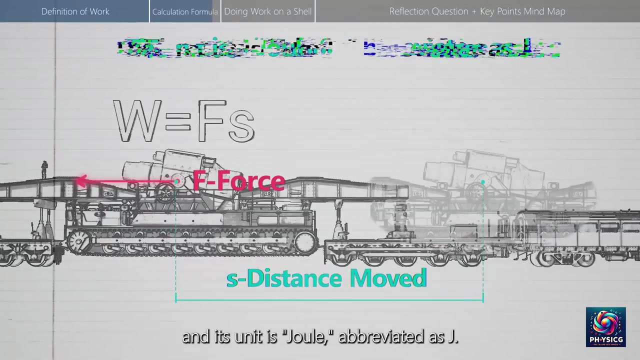 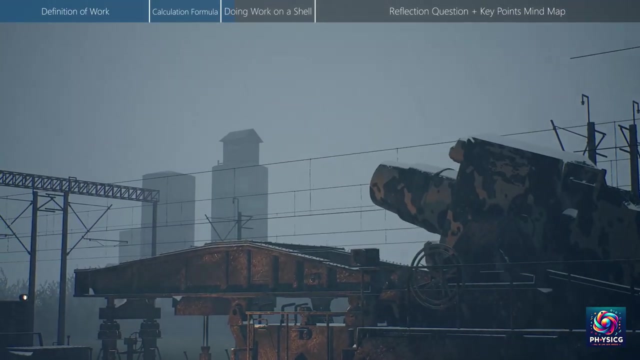 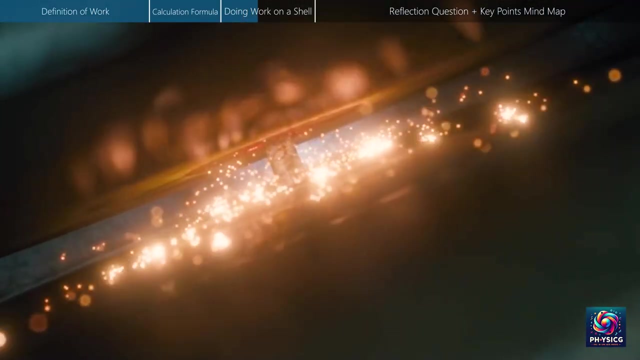 work on it. The formula for work is W equals FS. where W represents work, F represents the force acting on the object, S represents the distance the object moves And its unit is Joule, abbreviated as J. This is the power of the cannon. The explosive force also does work on the shell. 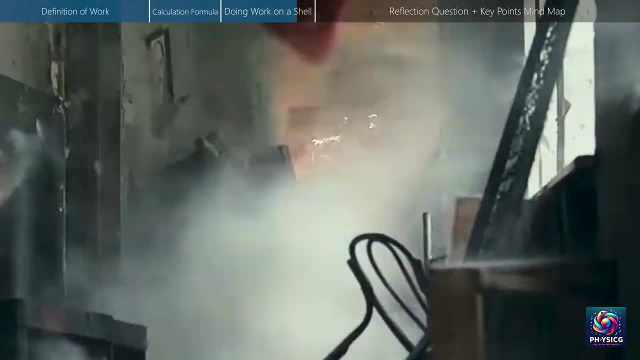 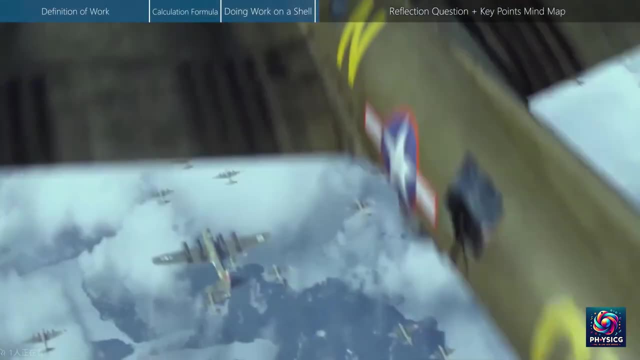 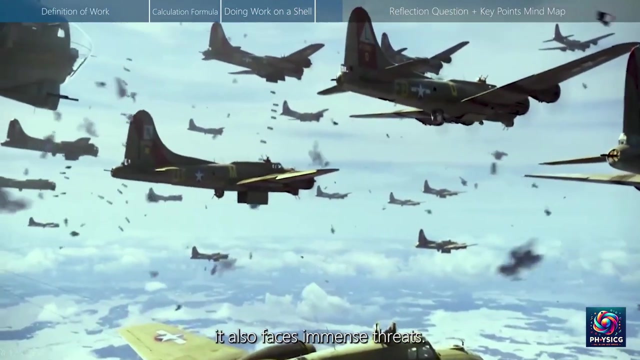 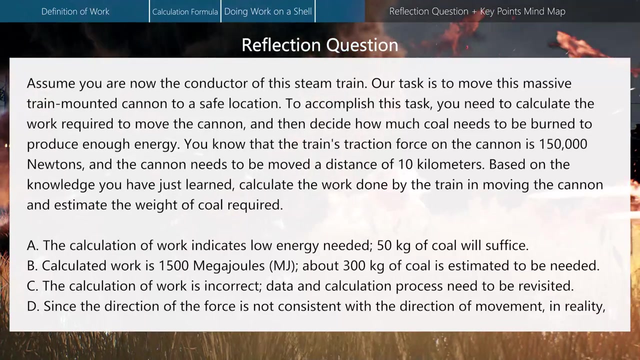 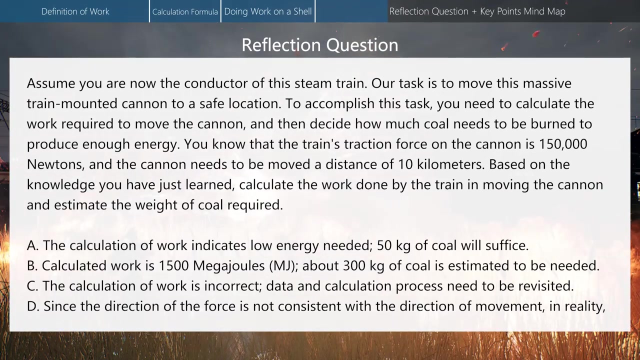 But on the battlefield it also faces immense threats. Emergency Students. assume you are now the conductor of this steam train. Our task is to move this massive train-mounted cannon to a safe place. To accomplish this task, you need to calculate the work required to move the cannon and 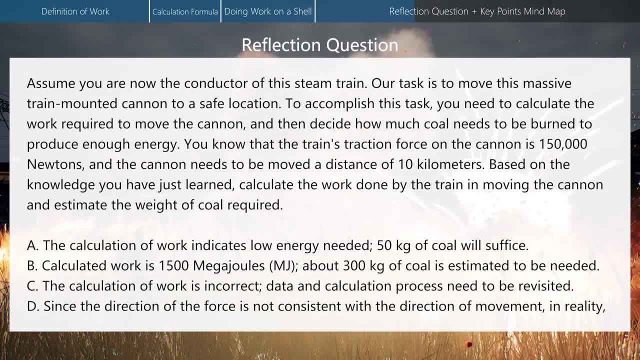 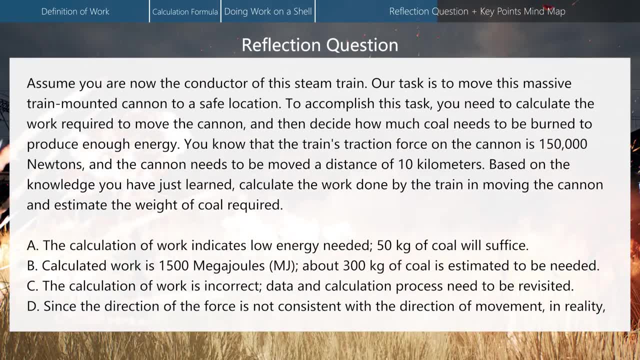 then decide how much coal needs to be burned to produce enough energy. You know that the train's traction force on the cannon is 150,000 newtons and the cannon needs to be moved a distance of 10 kilometers. Based on the knowledge you have just learned, calculate: 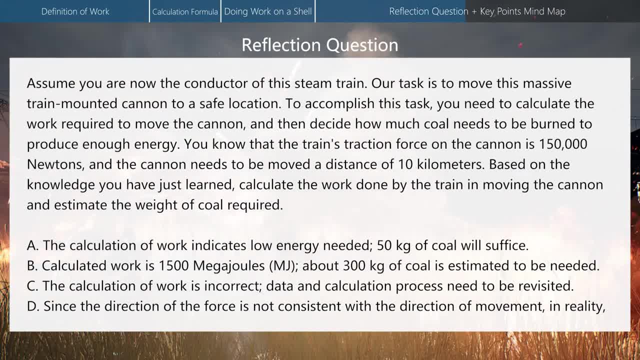 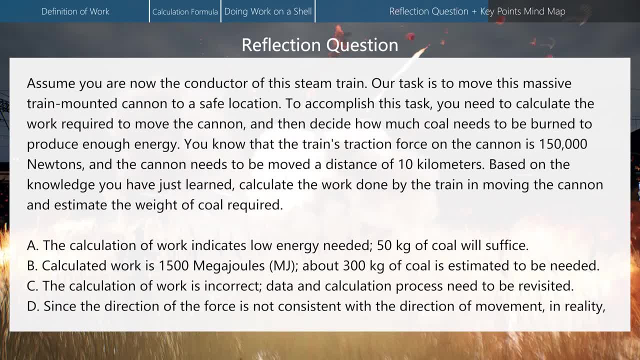 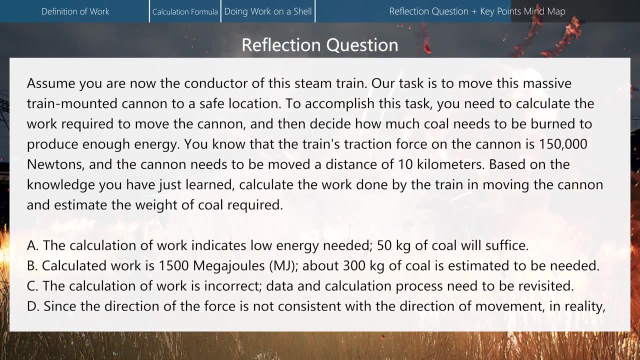 the work done by the train in moving the cannon and estimate the weight of coal required. A- The calculation of work indicates low energy needed. 50 kilograms of coal will suffice. B- Calculated work is 1500 megajoules. About 300 kilograms of coal is estimated to be needed. 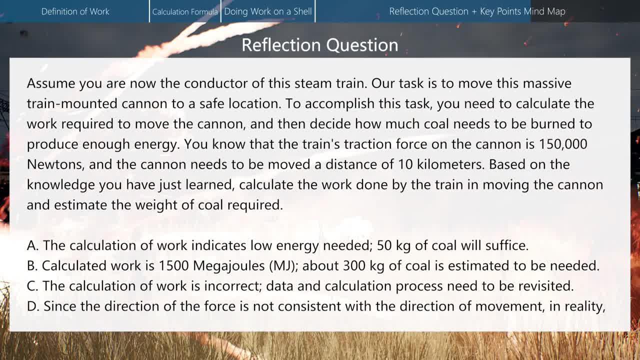 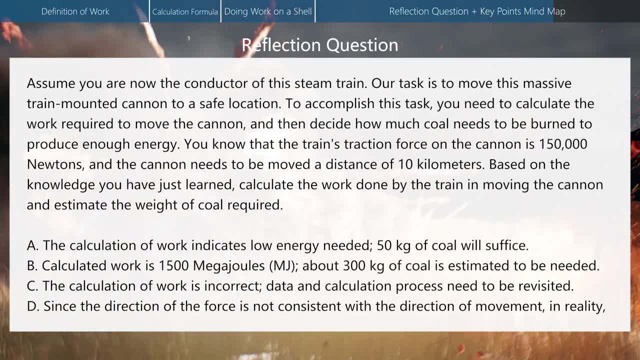 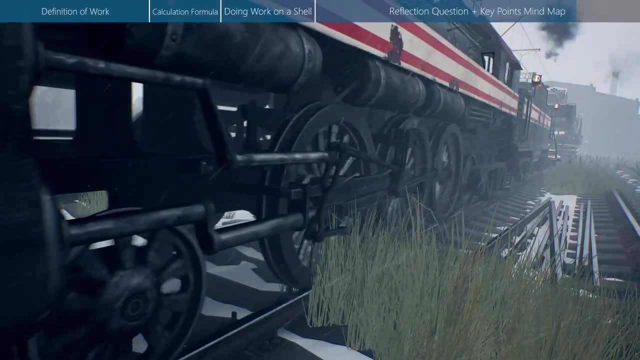 C- The calculation of work is incorrect. Data and calculation process need to be revisited. D- Since the direction of the force is not consistent with the direction of movement, in reality, no work is done. Consider using alternative energy sources. If answered correctly, the cannon will be successfully moved, avoiding bombardment. 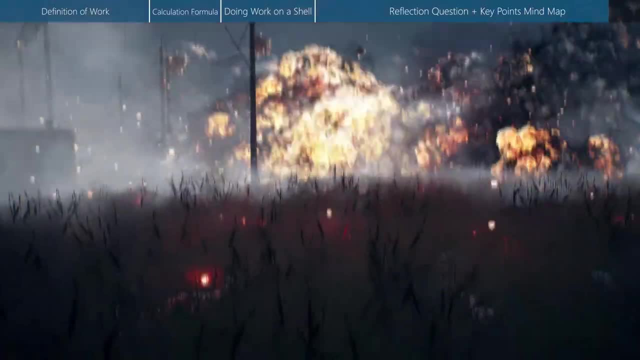 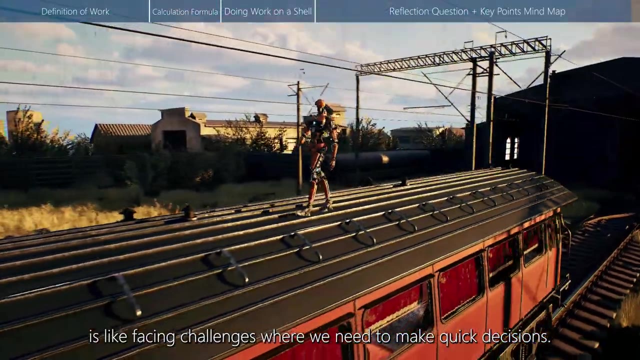 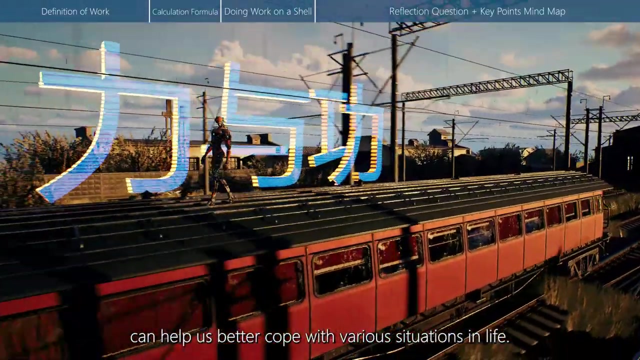 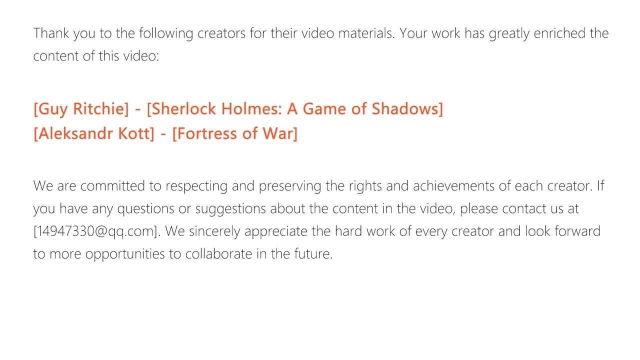 If answered incorrectly. the process of learning physics is like facing challenges where we need to make quick decisions. Understanding the relationship between force and work can help us better cope with various situations in life. Subtitles by the Amaraorg community.